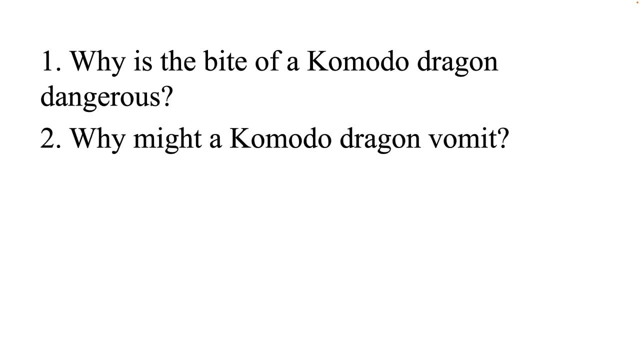 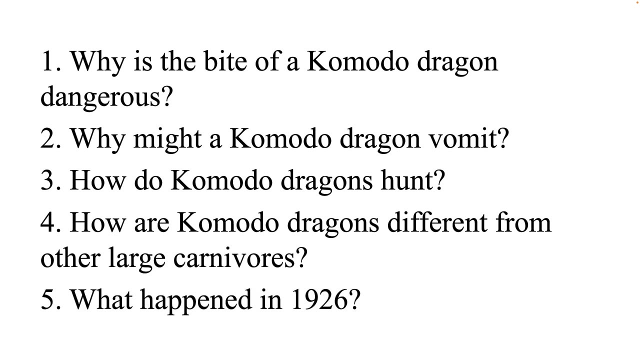 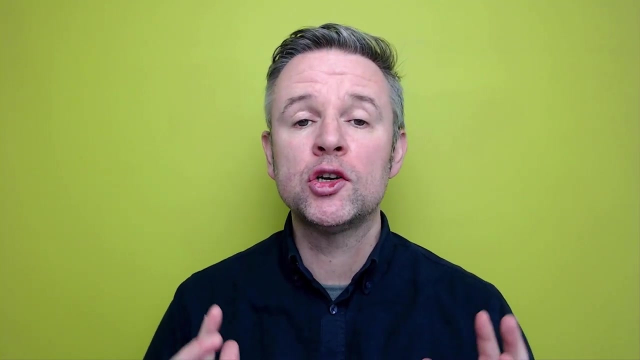 dragon dangerous? Number two: Why might a Komodo dragon vomit? Number three: How do Komodo dragons hunt? Four: Are Komodo dragons different from other large carnivores? And five: What happened in 1926?? Remember, the questions will be on screen. However, you might need a pen and paper to jot down your 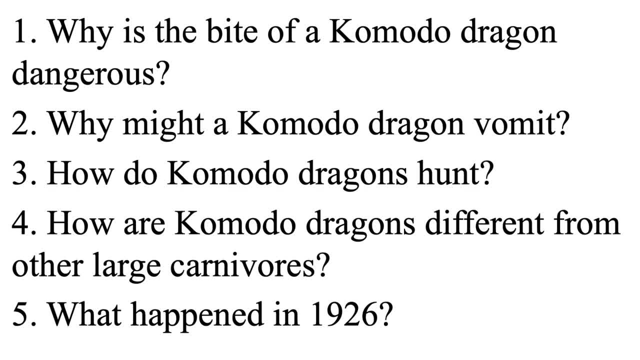 answers Ready, Let's begin. The Komodo dragon. Over three meters long, with extremely sharp claws, huge teeth and a poisonous bite. Although this may sound like something from a horror film, it is in fact a description of the Komodo dragon, These reptiles. 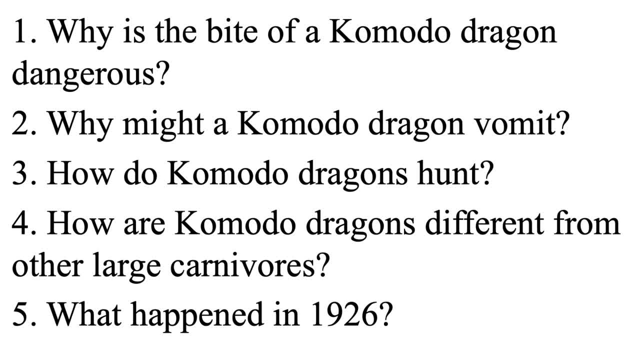 are real and they are one of nature's most incredible creatures. Komodo dragons have lived on some of Indonesia's islands for thousands of years. One story tells that the Komodo dragon was first discovered during World War I, when an airplane crash landed in the waters around the 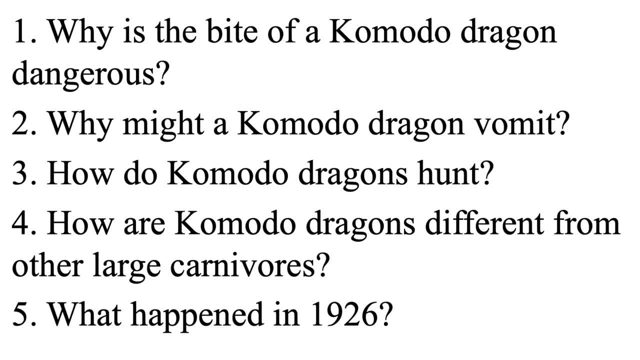 islands. The story tells how the pilot swam to Komodo island, where he was surrounded by a terrifying huge lizard. It sounds like something out of an action movie. However, the story is actually a myth. We don't know exactly when Komodo dragons were first discovered, But the earliest stories 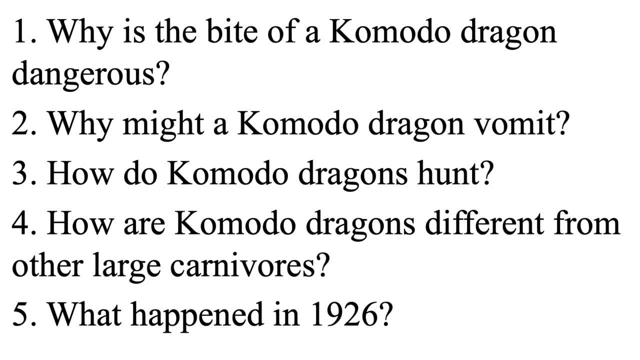 come from between 1910 and 1912.. The existence of the Komodo dragon was confirmed in 1926.. This was the year that the explorer W Douglas Burden led an expedition to Komodo. He was working for the American Museum of Natural History. He returned from his trip with twelve. 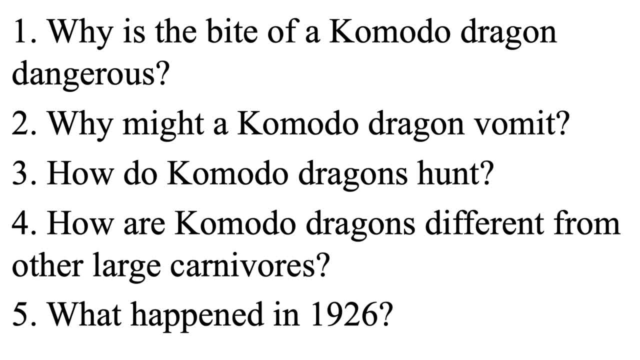 dead specimens and two living Komodo dragons. The Komodo dragon is the largest living lizard in the world. Some Komodo dragons can be 3 meters long and can weigh more than 130 kilograms. This means that the Komodo dragons are the heaviest lizards on Earth. They have long heads with short snouts, scaly skin, short. 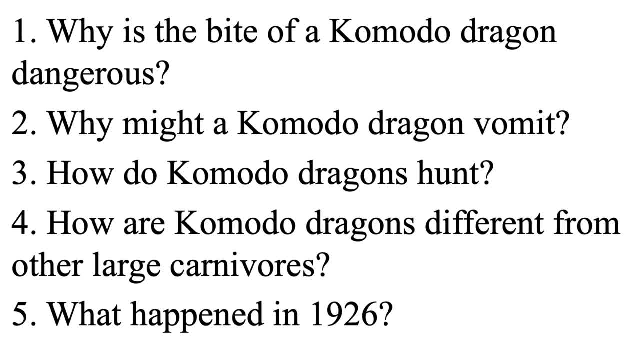 legs and big, strong tails. The largest dragon ever found was 3.13 meters long. This scary long and weighed 166 kilograms. Komodo dragons are the top predators on the islands where they live. They will eat nearly anything, including carrion, small dragons, wild horses and pigs large. 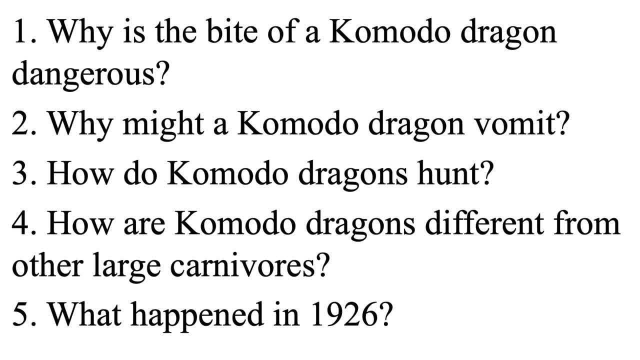 water buffalo and sometimes unlucky humans. Although the Komodo dragon can run briefly at 20 kilometers per hour, the reptiles usually hunt using camouflage and patience. They can spend hours in one place waiting for their prey. When their unfortunate victim passes, the dragons attack and rip it to pieces. 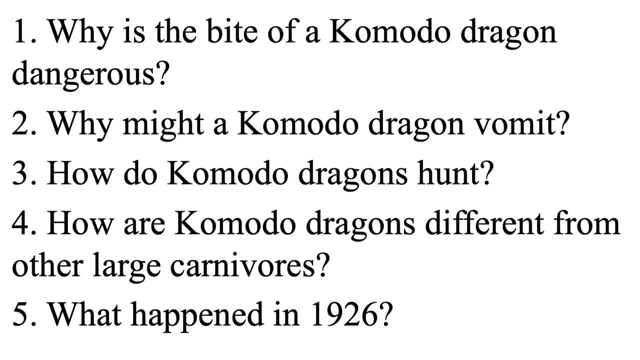 Komodo dragon saliva has more than 50 types of bacteria. If the prey animal is bitten and escapes, it usually dies of blood poisoning quite quickly. If this happens, the dragons follow and locate the dead or dying animal by using their excellent sense of smell. 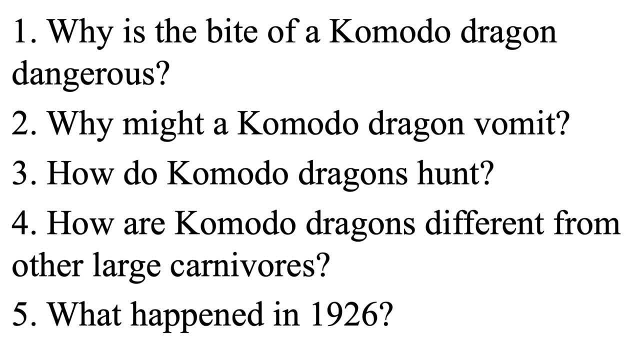 Many large carnivores, such as tigers, do not have a sense of smell. They do not eat 25 to 30 percent of their prey. They leave the stomach, hide, bones and feet. However, Komodo dragons are less wasteful and leave only about 12 percent of their prey. 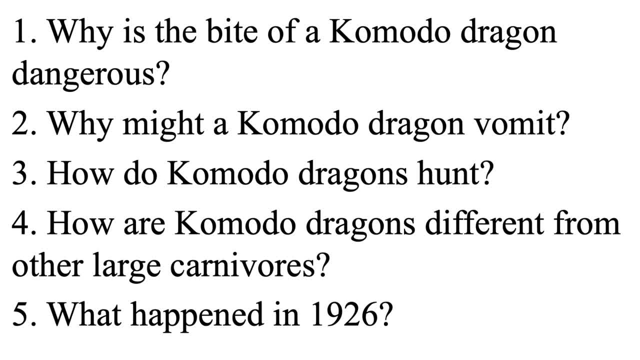 They eat bones, feet, fur and skin. They even eat the stomach. A Komodo dragon can eat 80 percent of its own body weight. However, when they feel scared or nervous, Komodo dragons can throw up the contents of their stomachs. 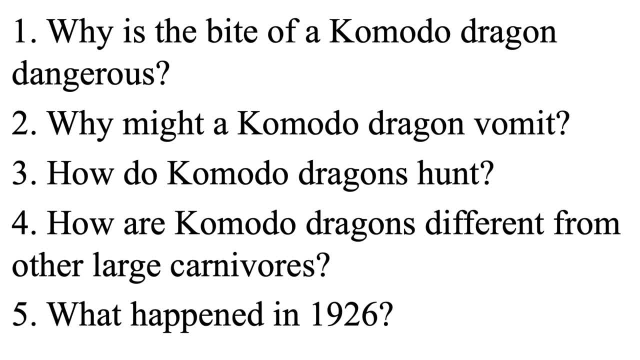 This makes them lighter, so they can escape more easily. There is a population of roughly 4,000 Komodo dragons on the island of Komodo. in the smaller surrounding islands, However, the species is endangered due to hunting, natural disasters such as volcanic. 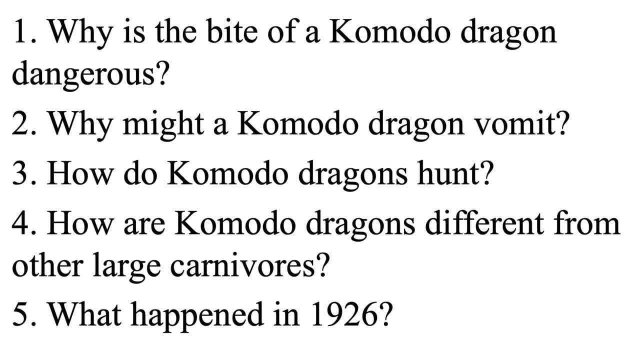 eruptions, forest fires and human expansion. Komodo dragons have always been popular in zoos around the world. Visitors love their huge size and scary reputation. Nevertheless, they are quite rare in zoos. Komodo dragons are a rare species. 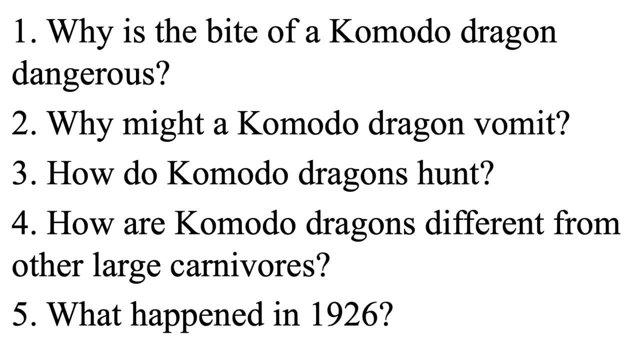 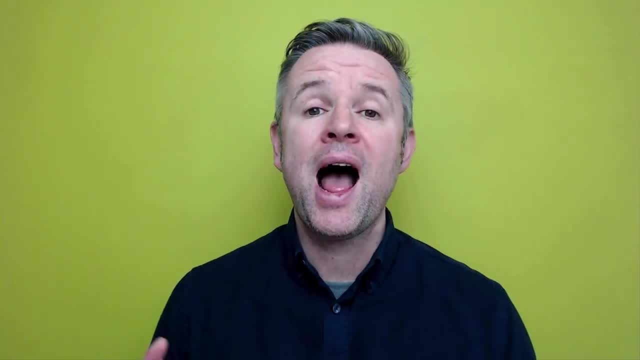 They are vulnerable to infections and parasitic diseases. Despite all that we have discovered about these magnificent creatures in the last century, we still have a great deal to learn. Who knows what secrets these amazing reptiles will reveal in years to come? I am now going to share with you the answers to each of the five comprehension questions.